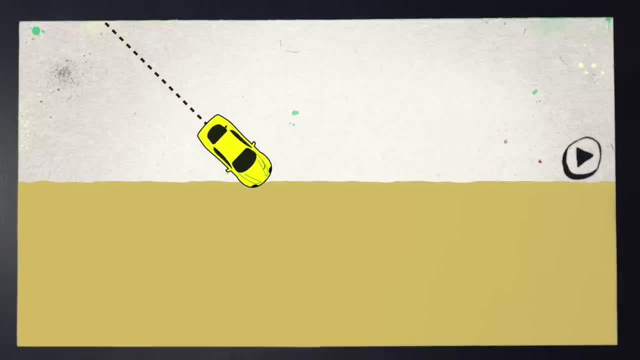 the car reaches the sand at an angle. As the first wheel reaches the sand, it slows down, But for a short period of time. the other wheels continue at a faster speed Because the wheel on one side is going slower. the whole car turns slightly. Once the whole car 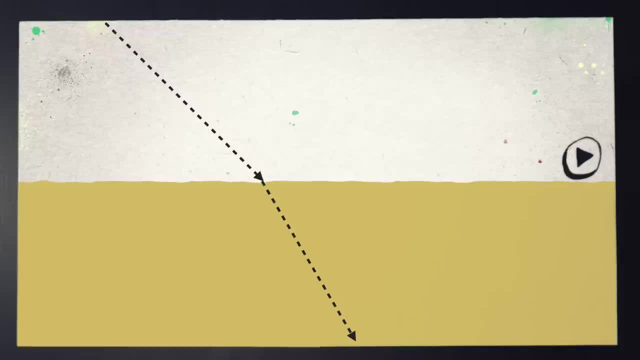 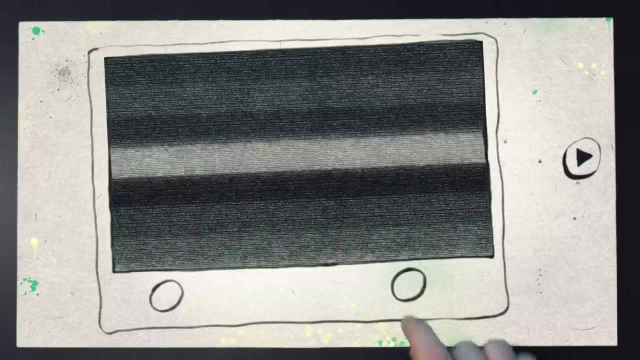 is on the sand. it continues in a straight line, but not the same straight line that it was travelling on along the road. Light rays work in the same way. If light rays are moving through air and reach a different material at an angle, they'll change direction slightly. 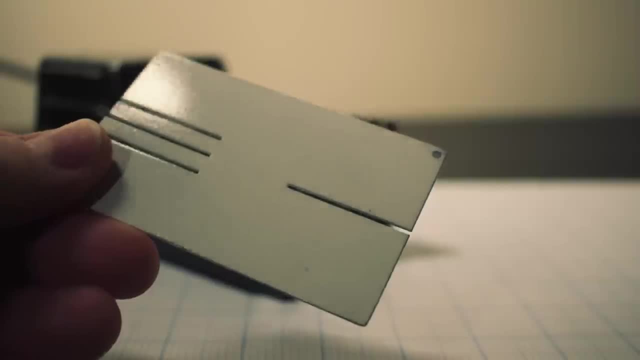 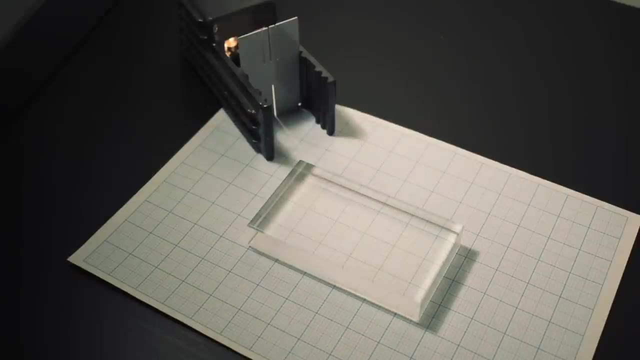 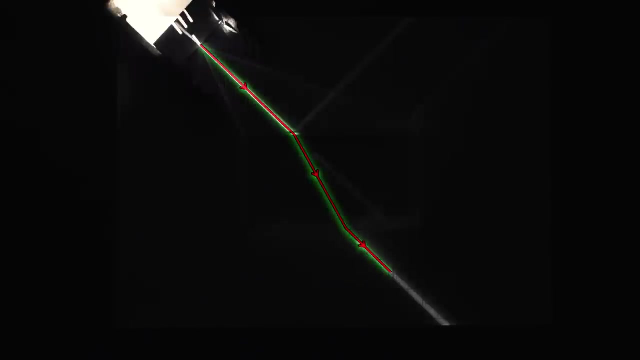 This is a ray box that we often use for light experiments, And this cover lets us beam a narrow ray of light from the bulb. If I aim the beam at the plastic block at an angle and turn the other lights in the room off, you can see the light beam is bent as it enters the plastic and again as it. 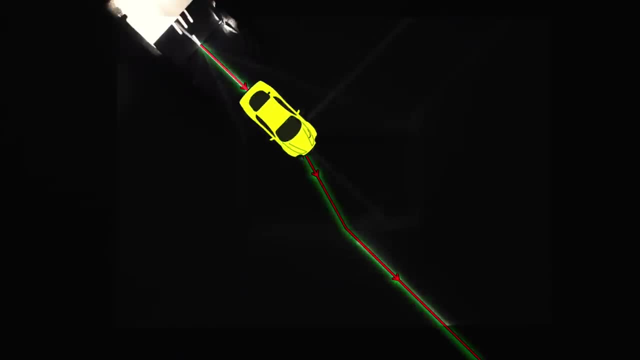 exits. This happens just like the car reaching the sand. The speed of the light ray decreases as it reaches the plastic block, but then speeds up again as it exits the block. This bending of light is known as refraction. We can say that the light is refraction. 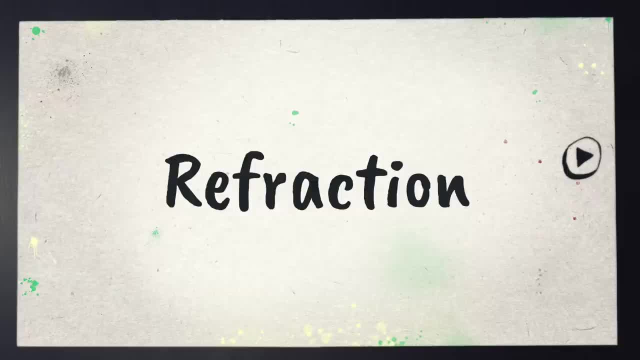 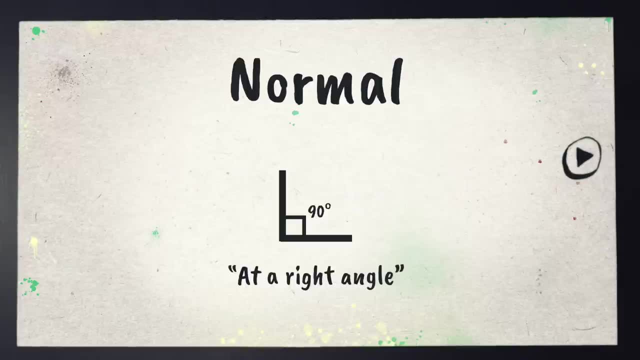 Let's consider some of the details of what we're observing. First, you need to understand the word normal. Normal is a word that comes from latin, meaning at a right angle. The normal is an imaginary line at a right angle to a surface Looking. 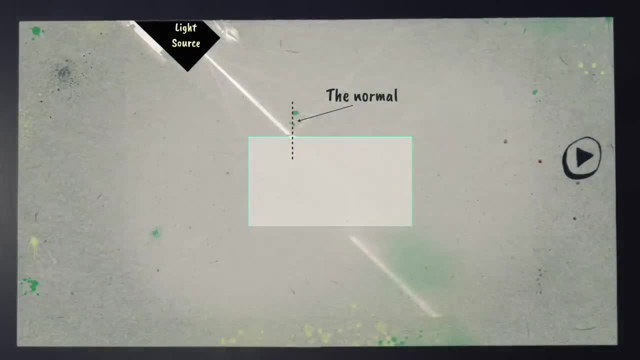 at the ray box setup. here you can see the normal drawn at a right angle to the surface of the plastic block, And when we talk about angles of reflection and refraction, we describe them relative to this line. Here The ray known as the incident ray reaches the plastic block at 45 degrees from the normal. 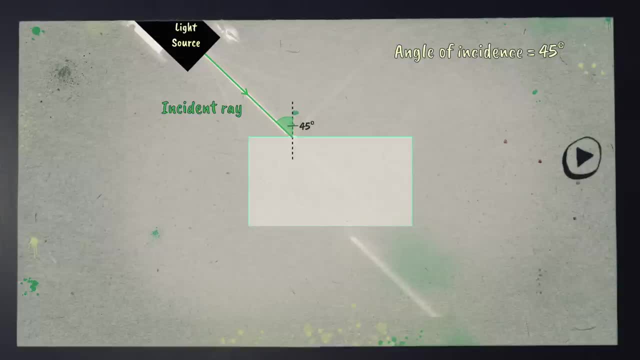 This is the angle of incidence. The ray within the block, known as the refracted ray, moves through the plastic block at 30 degrees from the normal. This is called the angle of refraction, Because the light then exits the plastic block and returns to air. it speeds up The emergent. 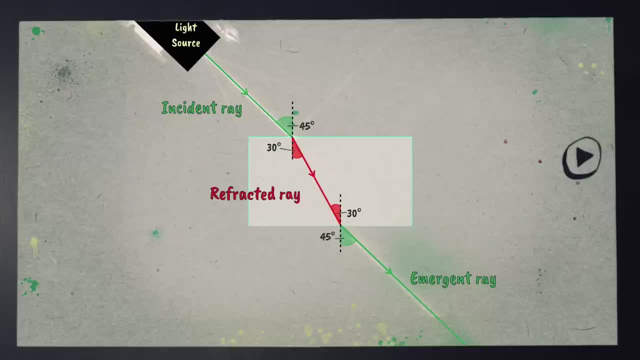 ray exits the plastic block at the same angle as the incident ray. This is called the angle of refraction. In a case like this, the incident ray and the emergent ray will always be parallel to each other. So how does refraction affect how we see the pencil in water?